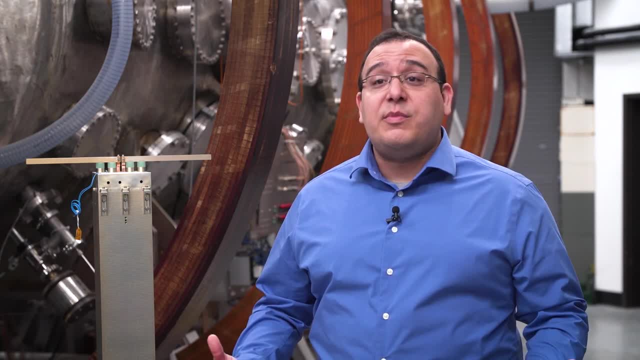 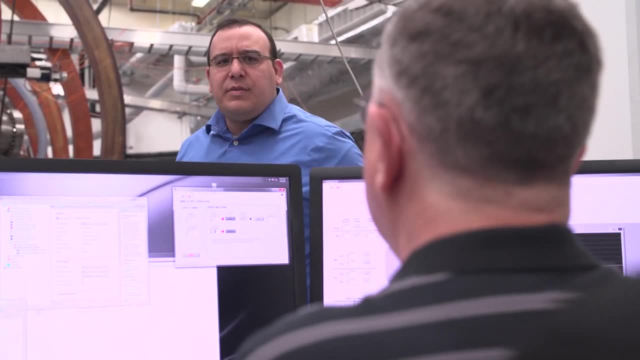 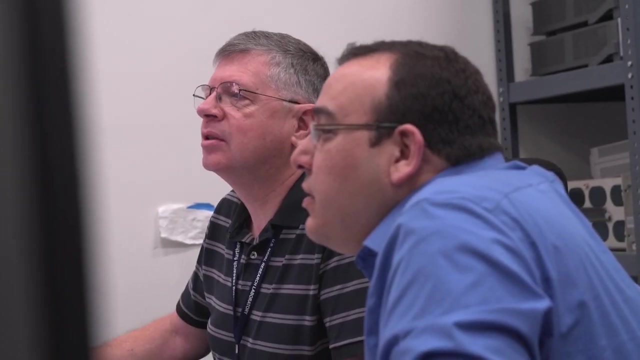 alternative to launching satellites and sounding rockets and making measurements in space. SPADE is a space diagnostic that was first started out as a laboratory diagnostic, where we're trying to measure background plasma parameters that are important as inputs to space weather models, but in addition can measure differential charging that can occur. 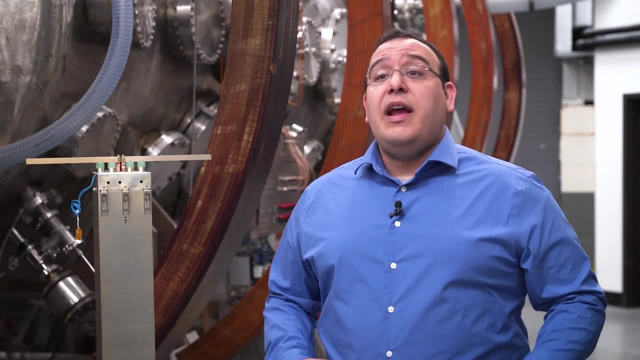 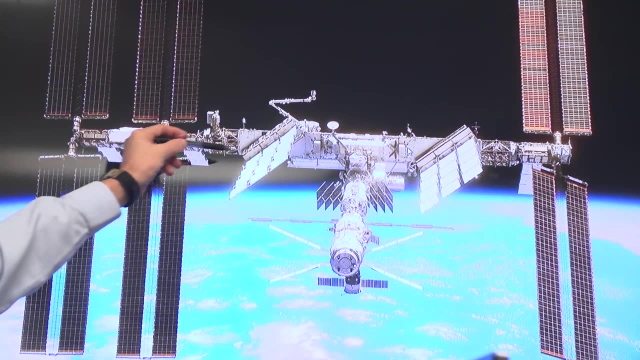 in spacecraft. So this has been tested in our laboratory here in the Space Chamber and now it's going to go up on as part of the SCPH6 pallets, a collection of instruments going to the International Space Station where we'll be able to test this diagnostic. 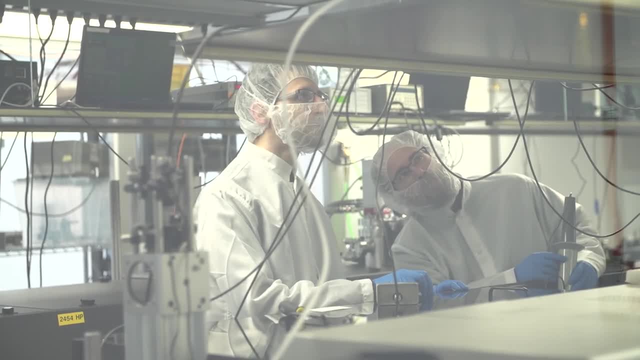 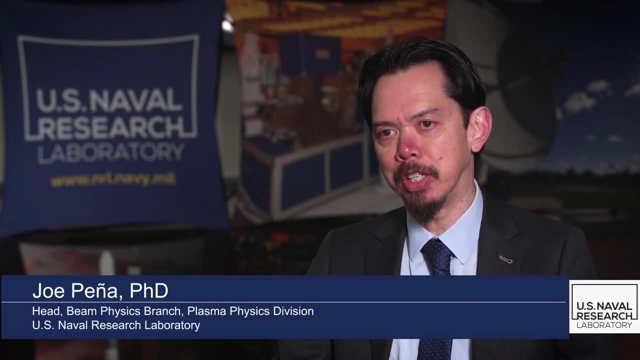 in a relevant environment. The NRL is a great place to do research. Scientists here are given free reign to pursue any kind of idea they have, if it has, if they can show relevance to not even today's Navy, but the Navy 20 years from now. 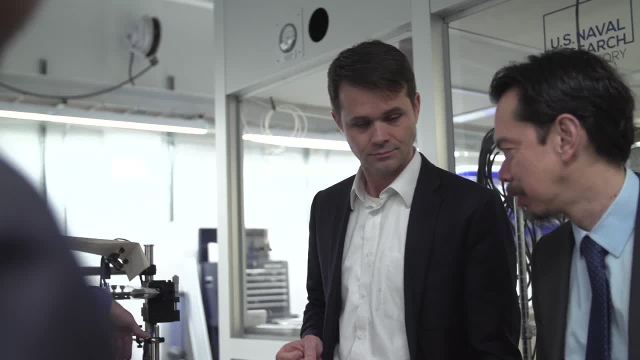 The Matrix Lab itself was a very unique experience. It was a very unique experience for us. It was a very unique experience for us. It was a very unique experience for us. It was a very unique facility here at NRL, What we've been working on for a number of years now. 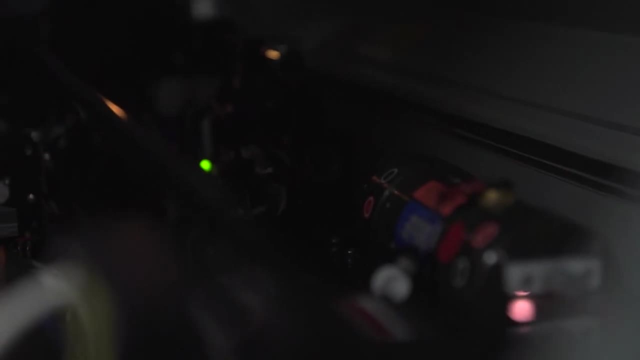 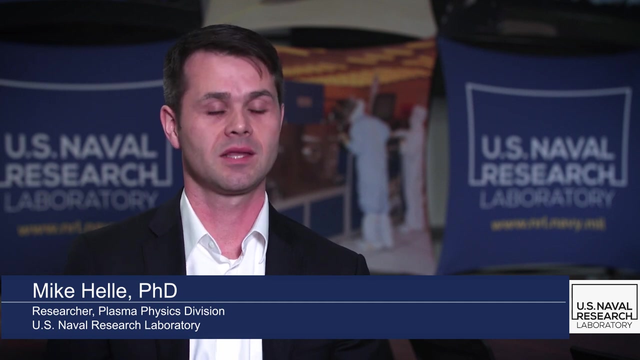 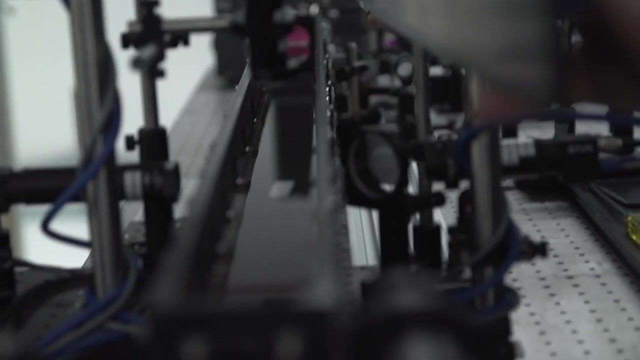 is bringing in a source where we can have very high intensity laser pulses that range all the way from the x-ray all the way out to the terahertz regime. At the same time that's synchronized to femtoseconds with particle beams, so that's ions and electron beams. 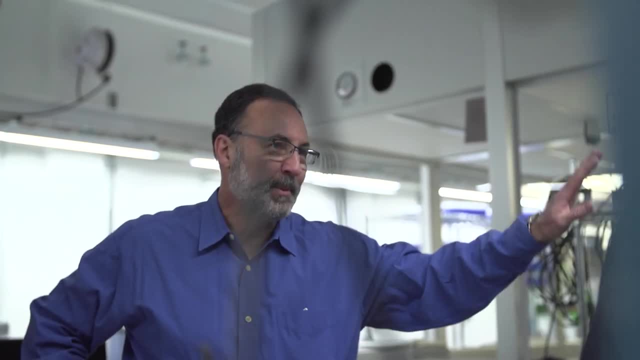 That allows us to do some really unique pump probe analysis of things like plasmas or other different materials that would be useful for the Navy. The Nike Laser at NRL is the world's highest-end laser. The Nike Laser at NRL is the world's highest-end laser. 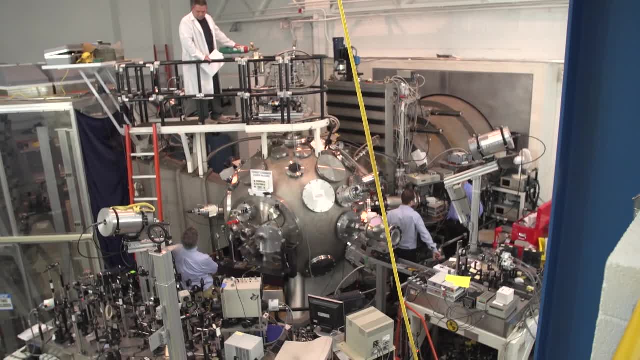 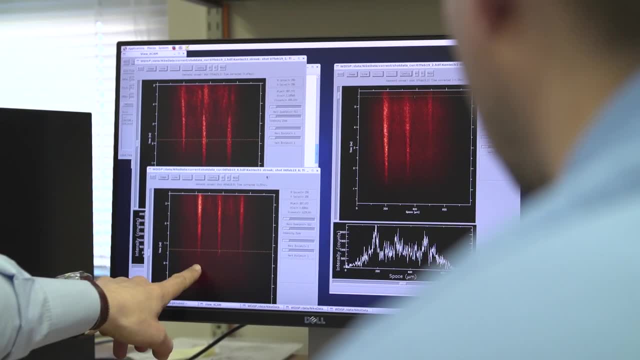 The Nike Laser at NRL is the world's highest-end laser. It's the world's highest-energy exmor laser, the world's deepest UV high-energy laser. It's a gas laser as opposed to glass laser, so it also has the potential for high rep rate operation. 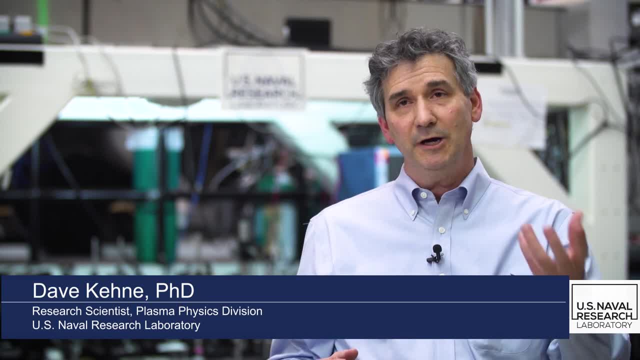 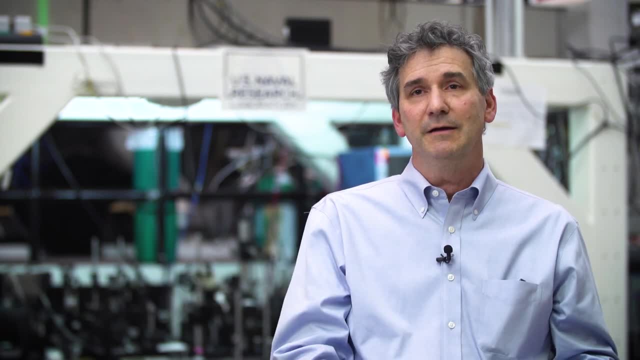 The facility basically focuses on two areas. There's the target issues, which are all the plasma physics and high-energy density physics that we like to that really the facility is devoted to studying. On the other side is the driver itself, which is the krypton. 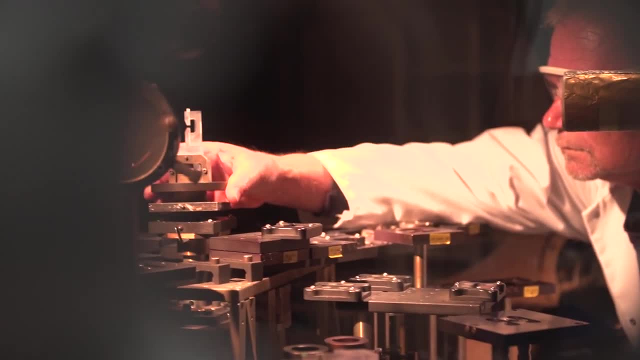 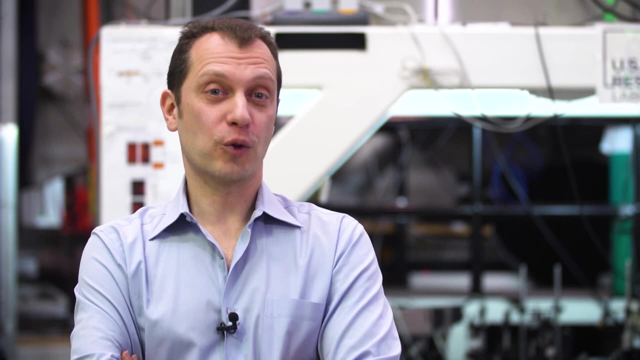 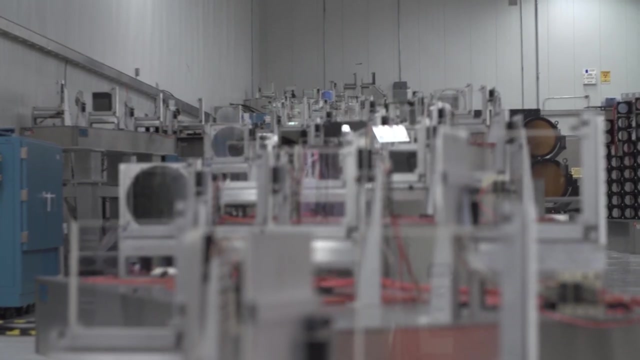 fluoride laser. So not only are we doing plasma physics experiments, we're also doing laser development work. The exmor lasers natively have a wider spectrum than high-energy lasers that have been used in the past. This technology seems to show large premise in helping suppress these deleterious 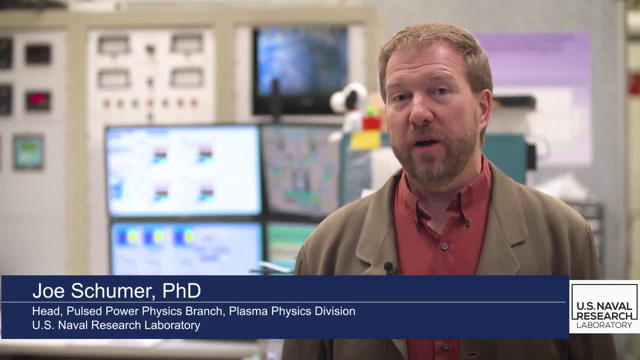 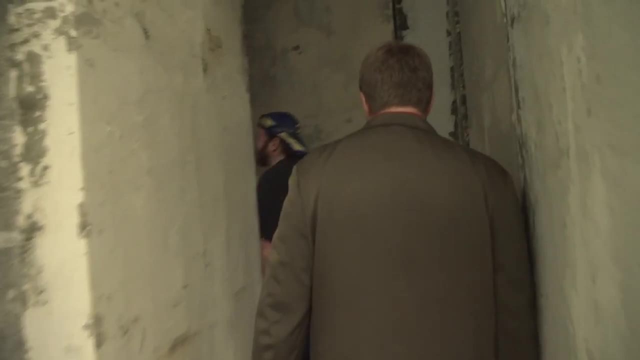 target instabilities. Our research with pulse power driven electron beams and ion beams is to support the Department of Defense and Department of Energy in various missions. Our bread and butter for our branch is the simulation of nuclear weapons effects, So we try to make the electron beams or the 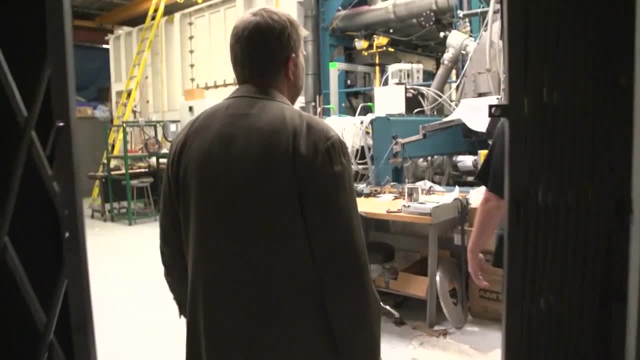 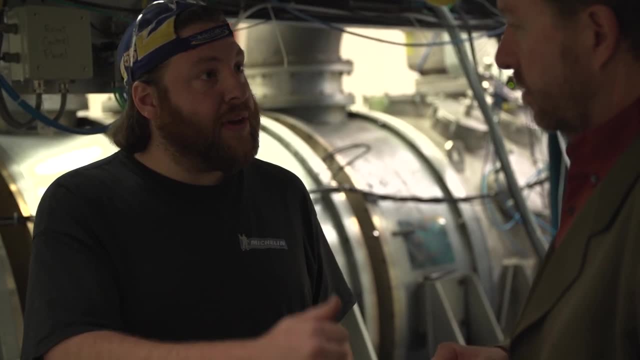 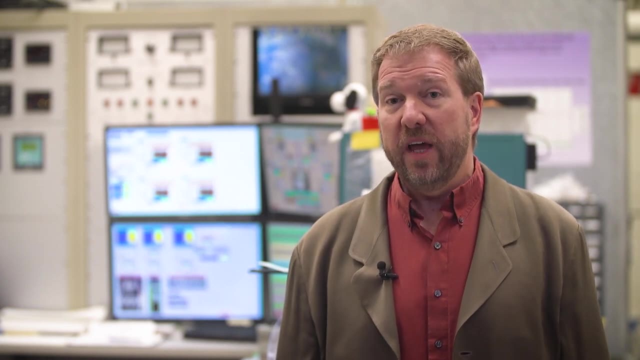 ion beams cleaner, better, stronger, faster to do the right mission. Our mercury accelerator goes up to about 8 million volts, 8 megavolts, but the current is 200 kiloamps. So we store up energy over many minutes timescale and discharge it over a few nanoseconds timescale. 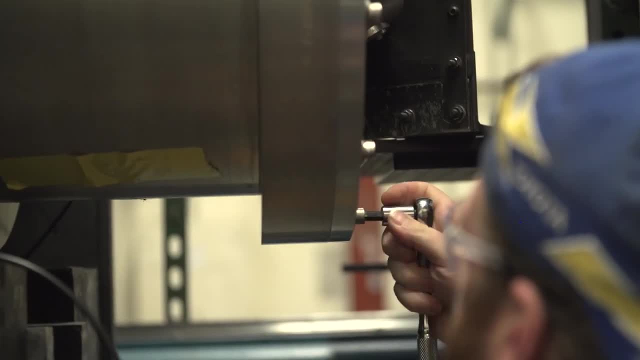 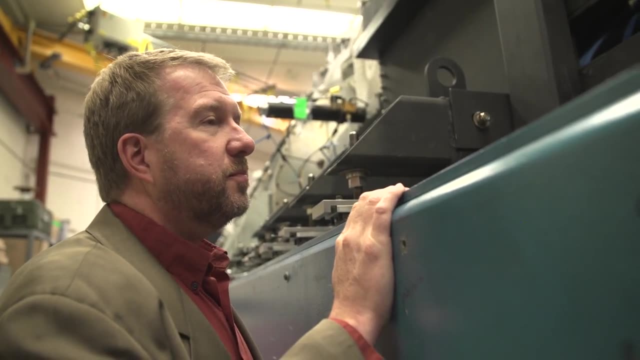 Another piece of the work that we do for electron beams and ion beams is to take X-rays, flash X-rays. We take very bright flashes of X-rays to take photographs of something moving, a dynamic material interaction, So explosives driving materials, and we take pictures and try to 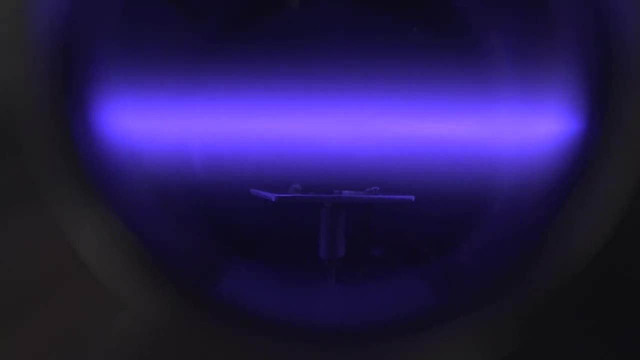 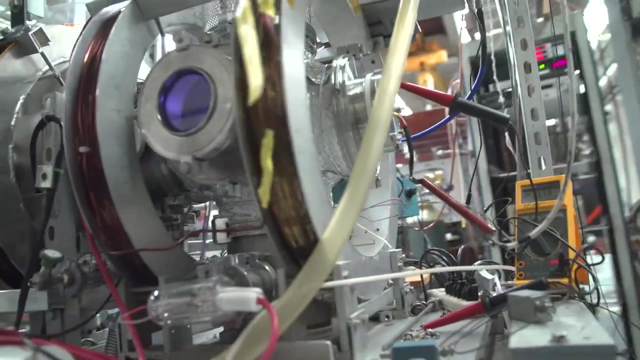 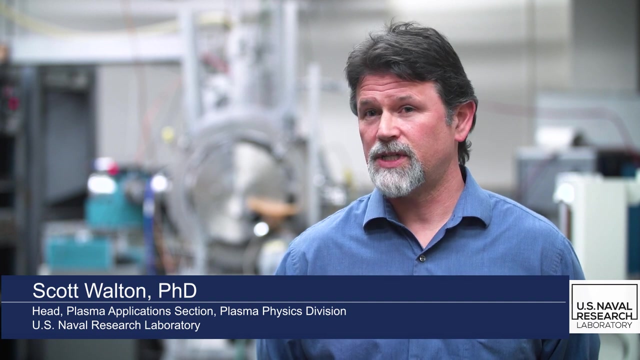 understand the physics of what's going on. In the plasma application section we look at applications where low temperature plasmas can be used to modify or process materials that are used in next generation devices. They can be low power or high power electronics. They can be used for sensors. Those materials 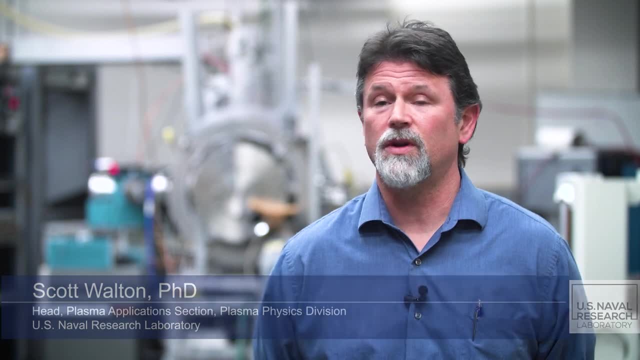 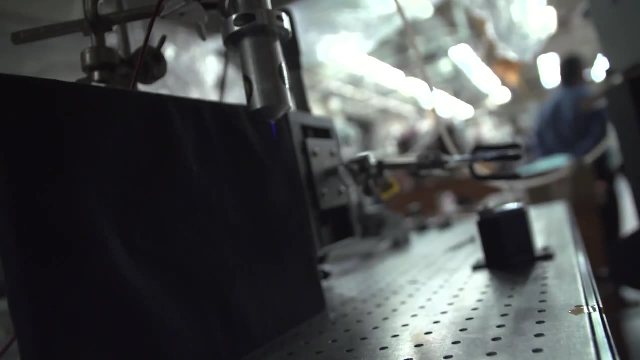 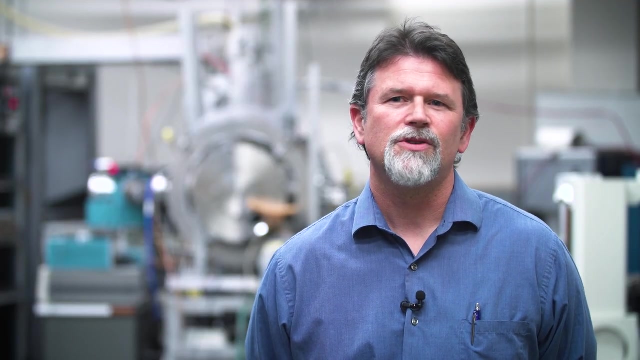 can be used as coatings. Coatings can be protective or those coatings can be adaptive in nature, And those various devices and coatings are typically used to advance the needs of our warfighter. Science by nature is pretty organic, so it's sometimes hard to predict where science will go. But 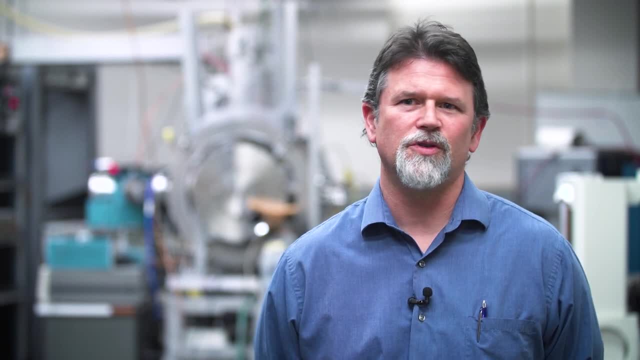 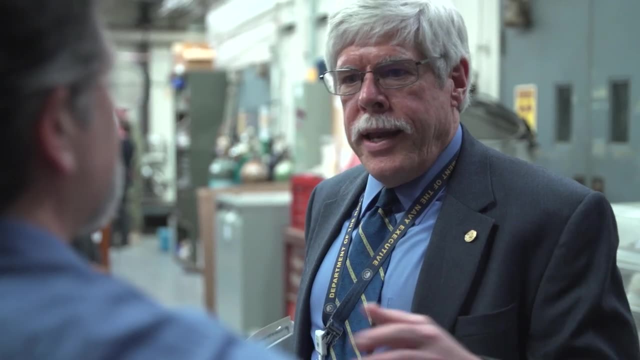 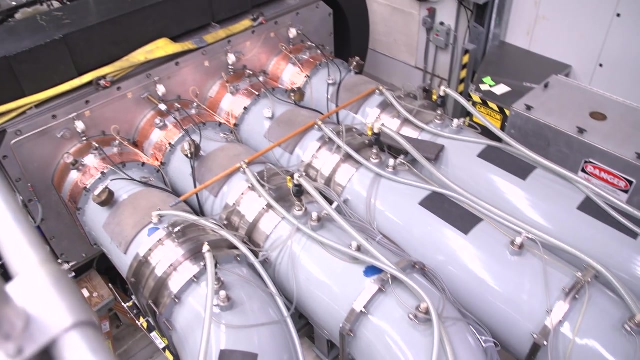 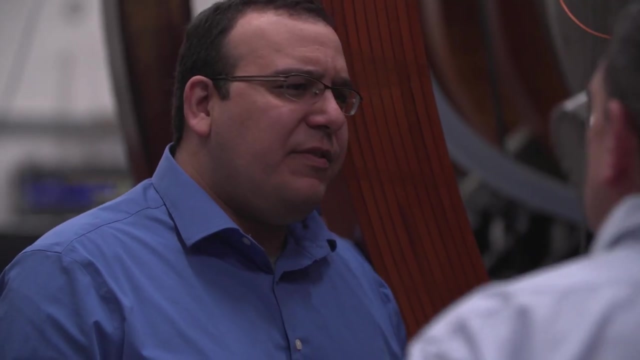 what I think the division will do is use those creative ideas and innovative ideas to continue to address serious problems that we have. Plasma physics has, in the last 50, 60 years, has become a discipline that touches everyone's lives, From advanced electronics to space weather that impacts our ability to communicate. 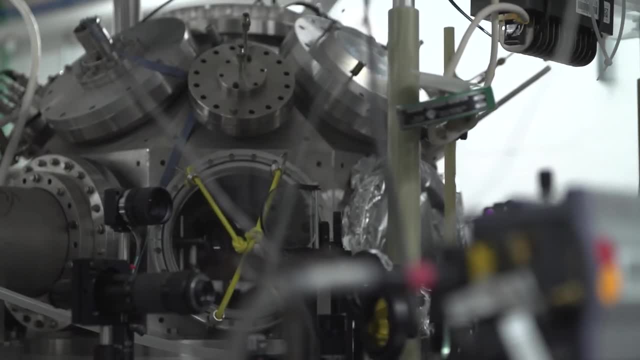 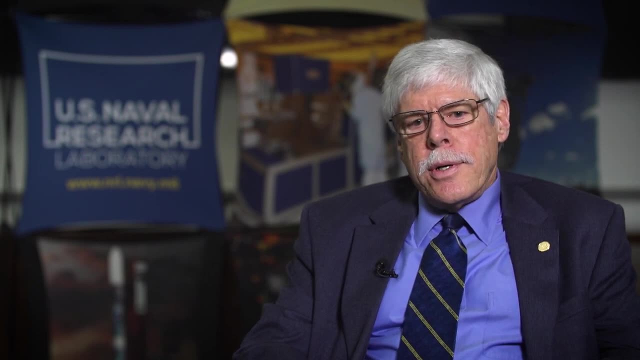 and navigate. So what I'm hoping to see in plasma physics is it becomes even more pervasive in the quest for new knowledge and new technologies. It's going to encourage new applications in this endless frontier of science.